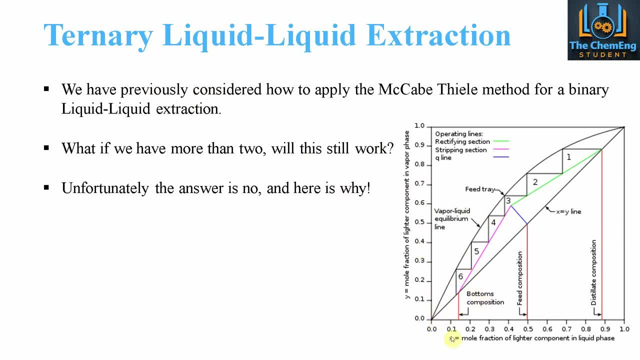 Because in terms of what we actually have is we have the mole fraction of the lighter component within the liquid phase and the mole fraction of the lighter component in the vapour phase. So here we only consider the x-y plot of one of the compounds in their respective states. 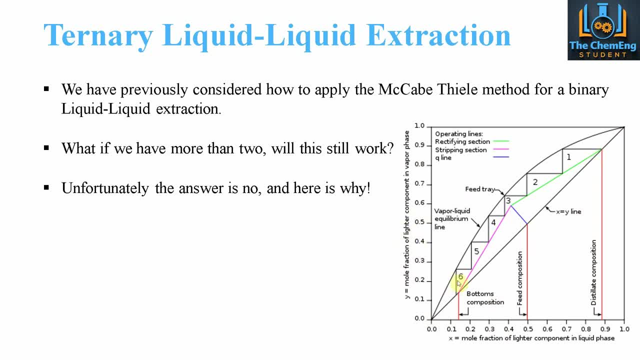 The other is the reciprocal. So here we consider the feed, we consider the distillate and we consider the bottoms. Because if we know that, say, for example, this is 50% of the lighter component, we assume that it's 50% of the heavier component as well. 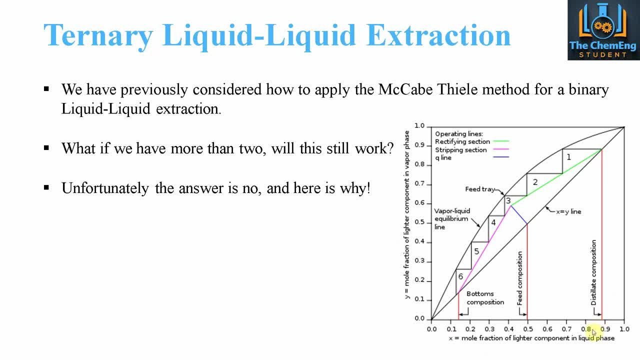 Likewise. imagine this was 90% of the lighter component, we would know the reciprocal is 10% of the heavy. Now the construction of the tie lines and the queue lines is pretty much going to be the same thing. So the question is: what is the solution for a ternary liquid-liquid extraction? 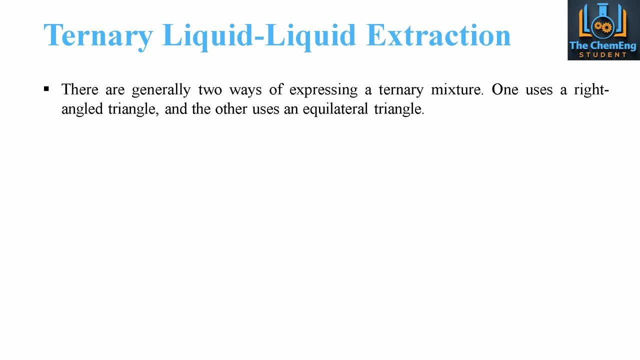 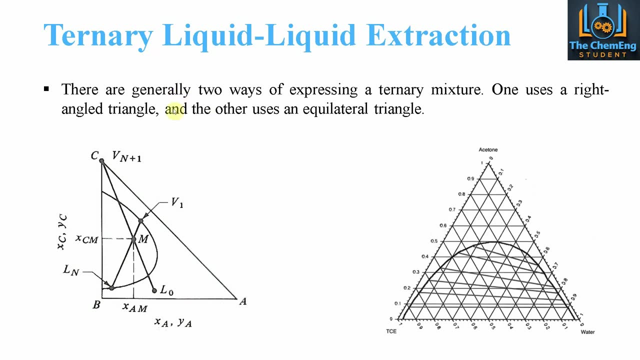 Then there's generally two ways that we can express this. One applies a right-angled triangle and the other one uses an equilateral triangle, And these tend to look something like this: Now we'll talk about the details as we go through this video, so we'll understand every. 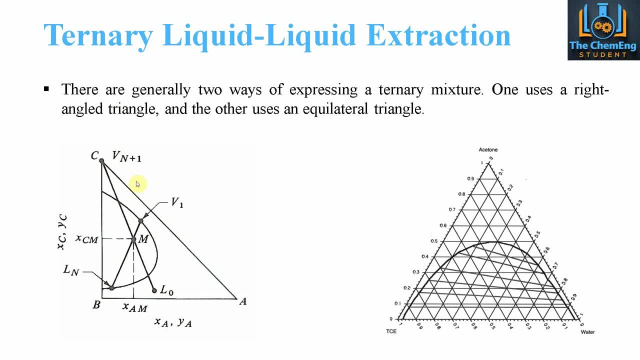 single variable, and then we'll look at a full working example so that it is very clear how you actually apply it. So let's go through this. So the first thing that we can notice here is on both sides and we're going to call. 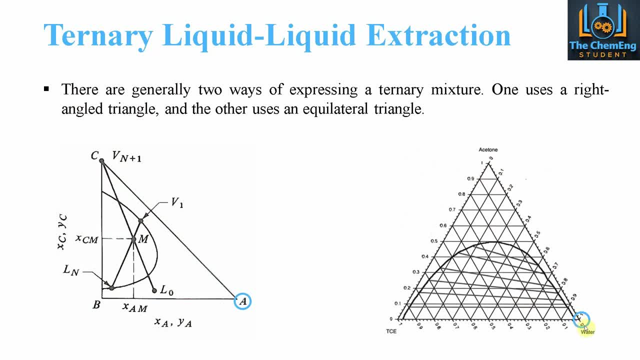 this one for a specific system. This is for the water and acetone and a TCE which is the trichloroethane molecule. So here we're going to call the water component A. So what this means is that we will highlight. 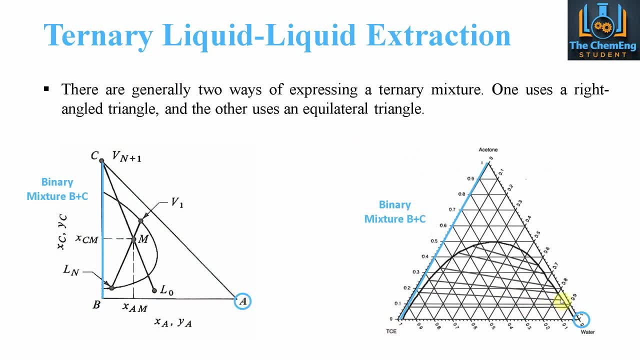 that at component A on both sides. So what this means is that we will highlight that at component A on both sides. we're going to call this one for a specific system, So let's go through this. So, if we look at both of these graphs, the opposite line indicates a binary mixture between: 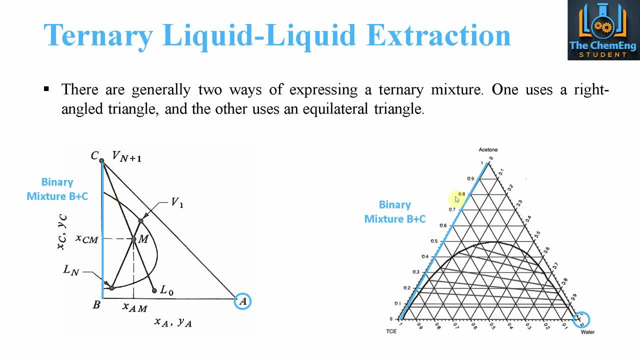 component B and component C, Because at this stage here we have pure, 100% water And here there is no water within the system. so we only have two components, ie a binary mixture, And it's the same thing here. 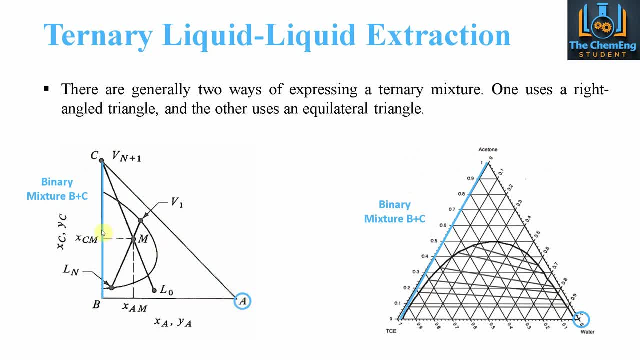 If this is pure A, then by the time we get to this point there is no A left, And that's echoed throughout the entire graph. So say that TCE is component B. then that means that the line directly across from it is a binary mixture, or, in this case, of pure A and C. Likewise, exactly the same thing. 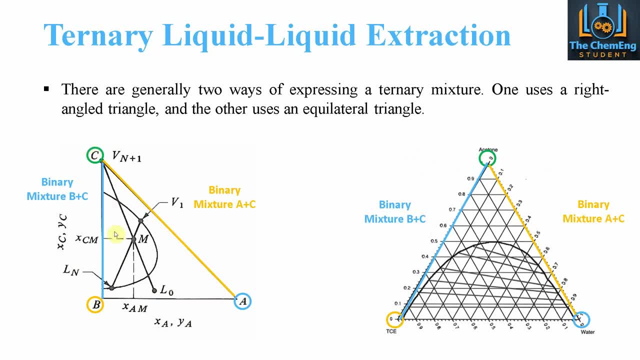 And then again, if we look at component C, then the line directly opposite would be a binary mixture of A and B, ie there is no C at this point. So if we look at component C, then there is no C at this point within the system. 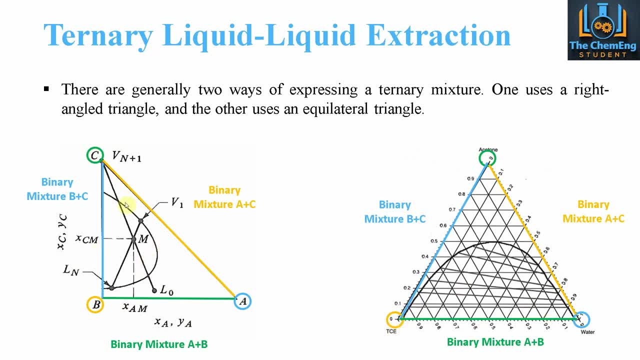 Likewise right here. Now, this one is slightly more simplified compared to this, but the general principle still stands in that we have this curve here and we have this curve here. So again, the system is pretty much exactly the same, but for this we get a more comprehensive 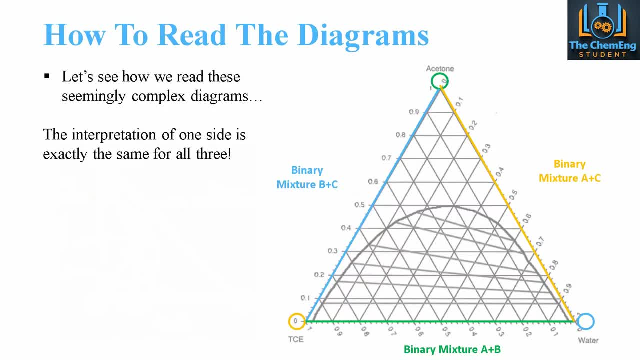 idea of the concentrations. Now, in order to actually read these graphs, we need to know what their concentrations are. So, in order to read these graphs, I'm going to use the more comprehensive one, but you can apply this to the right angle triangle as well. 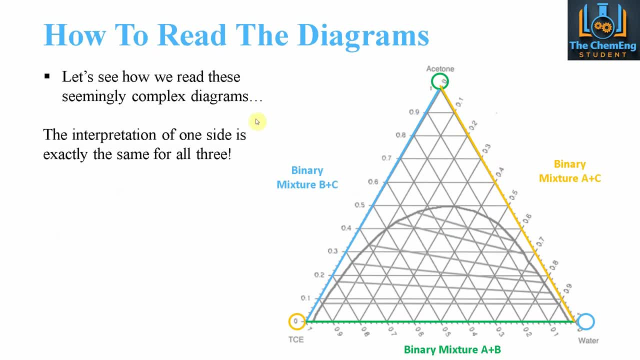 Now the interpretation of one of the sides is exactly the same for all three, So how we interpret one of the components is exactly the same for the others as well. So essentially, what we do here is as you move parallel from your respective axis. so 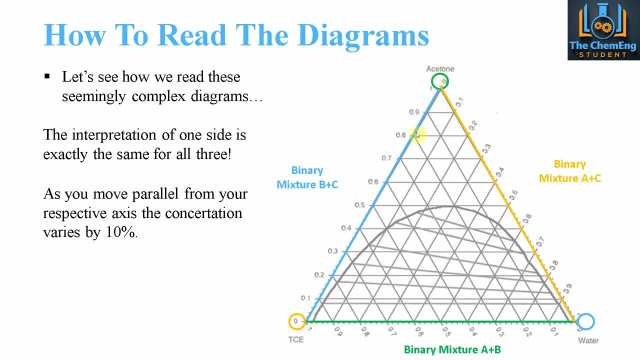 in terms of your respective component, Then in this case the concentration varies by a factor of 10%. So, for example, here that we have zero- sorry, pure TCE here. therefore, when we start to move from point to point, then the concentration begins to vary. 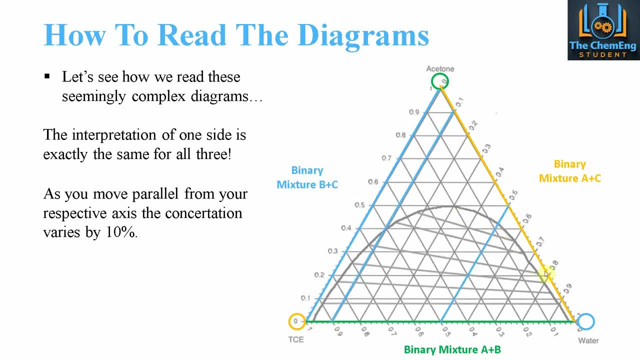 So what that means here is that in this case then, for the water system, we have no water at all. here, As we move further and further towards the water, our concentration increases by 10%, So that's on this axis. So here, at this point, we have 100% water. 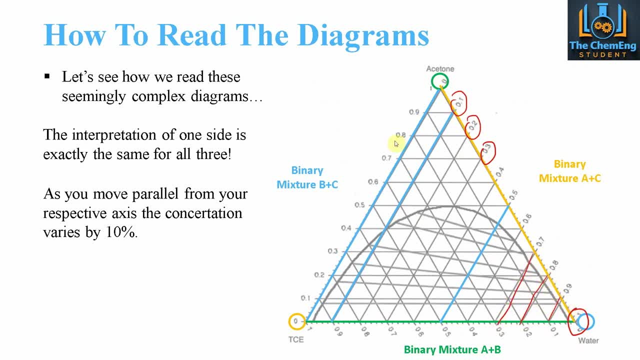 As we move on these diagonal lines, because, remember, it has to match the slope, it moves and gets closer to zero. Now, that's echoed throughout. So if we consider, Okay, The, the, the TCE, then at this point here we have a one, so that would be a hundred. 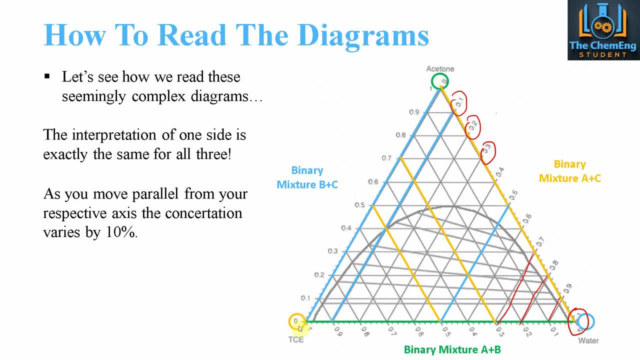 percent. But as we move away from the TCE, IE, as we head towards the binary mixture of A and B, then you can see that the concentration decreases by a factor of 10%. So these lines, as we travel away, we decrease by 10%. 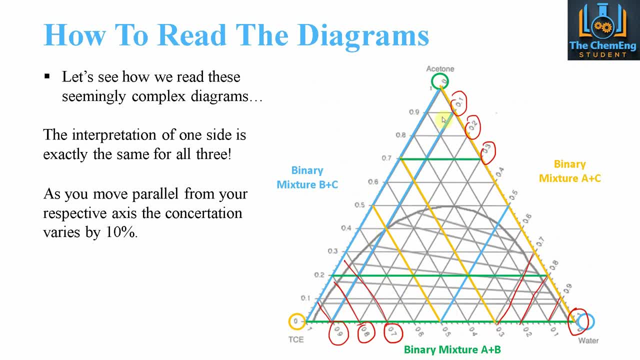 And then lastly the C, And then lastly the same thing with the binary mixture of A and B. So the acetone here is at a concentration of pure acetone, so 100%. But as we move away from acetone we can see that it gets less and less and less, up until 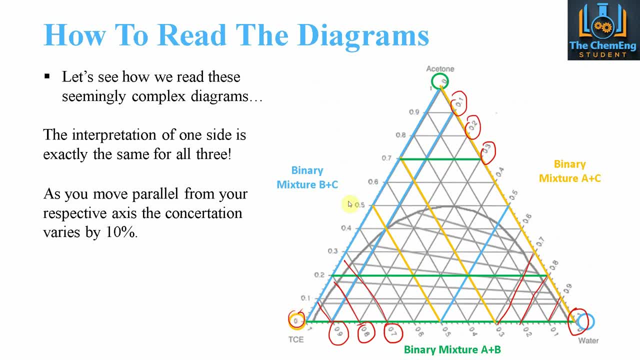 the point when the concentration is zero. So this line here is for acetone, This line here is for TCE. And then, lastly, the same thing with the binary mixture of A and B, So the acetone here is at a concentration of pure acetone. 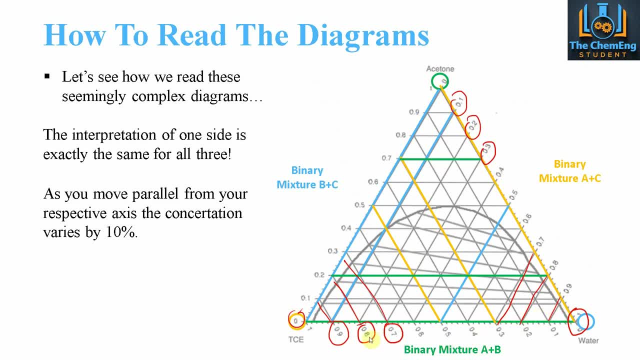 This line here is for TCE And this line here is for the water. So, again, you just need to make sure that your nomenclature is carried out correctly and that you remember that on the this type of graph, that we move in increments of 10%. 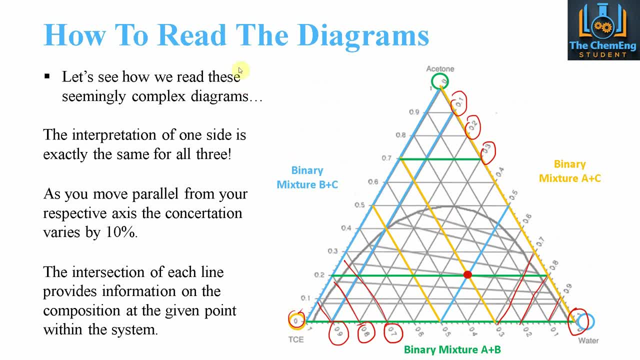 Now, the intersection of these lines would provide us with a composition at the given point within the system. So, for example, at this point here, Then what we would say Water is 50%, so a 50% water. We then, if we read down here, we have 30% in terms of TCE, which means the remaining. 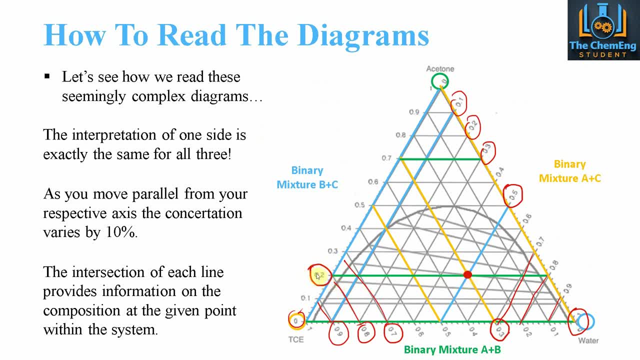 value would be point two percent, sorry, 20%. So if we do 50% plus 30% plus 20%, we can clearly see that we get a hundred percent. So that's what the makeup Of that point would be on both the streams- sorry, all three streams. Now the regions that we haven't. 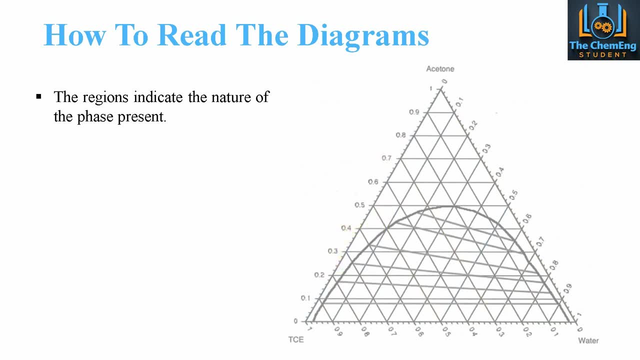 discussed, yet essentially represent the nature of the phases, because inside the curve, so we can express this as inside the curve, so that would be at this point, so this curve here, right, so inside the curve would be in this region. then what we have here is this: is the 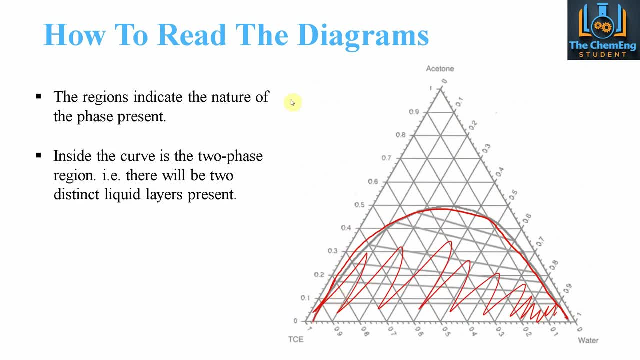 two-phase region, ie we would have two distinctive liquid layers, so kind of like you know, oil and water, how they would be immiscible with each other because TCE, so the trichloroethane and water, are completely immiscible with each other, so they will always. 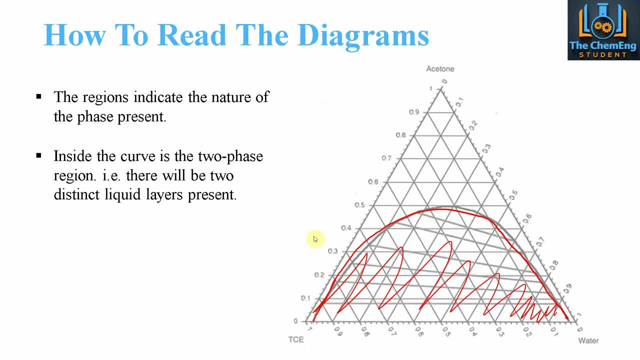 form a bilayer, so a two-phase region, whereas here in the outer region we have a single-phase region, ie we would have one single layer of liquid. Now, the single-phase simply means that, rather than having so here, if we draw this on a 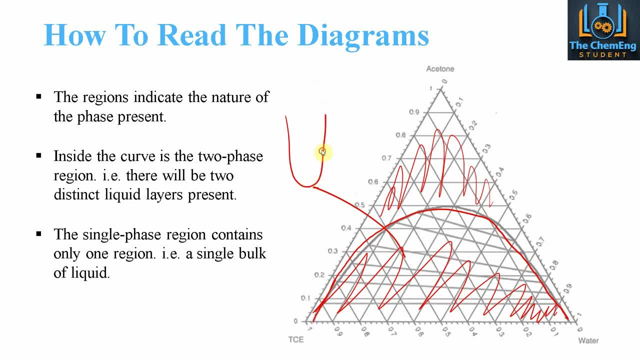 like a beaker. so the two-phase region would be: we have liquid one and we have liquid two. we would see the distinctive layer, but here what we would have is L1, L2 in the same batch. we wouldn't con. 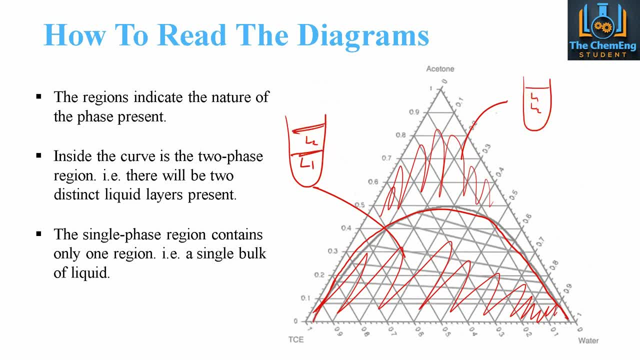 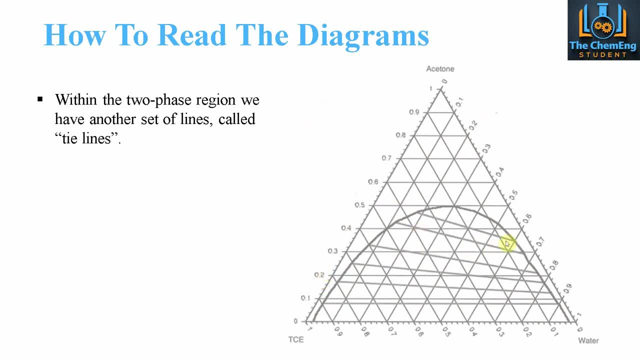 we wouldn't see this distinctive layer. so that's, that's the difference. Now, within the two-region, the two-phase region, we can now see we have these lines. Now these are called tie lines, and the tie lines give us information about the equilibrium. 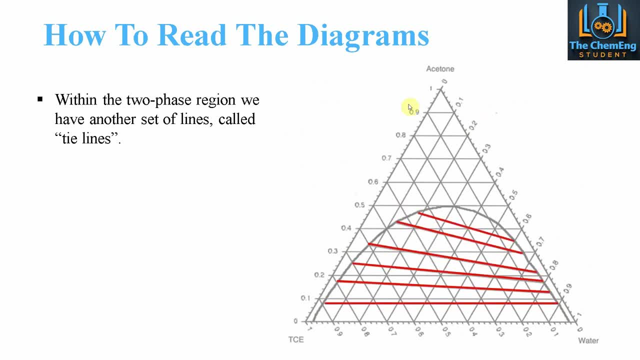 within the system. So that's all these lines here. Now there is a special point at this part here. so if you were to follow the lines as we gravitate towards the, the edge, when these points, you know, intersect, 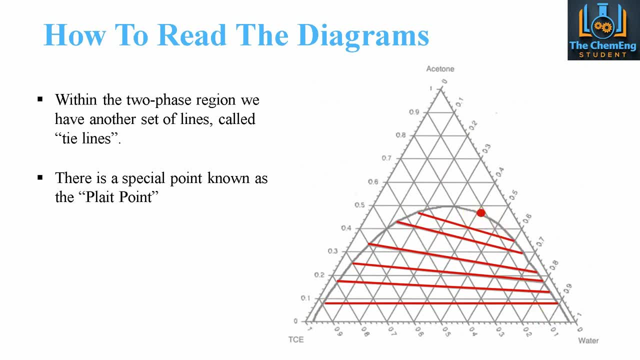 and converge where the, the turning points, basically become zero. then this is known as the plate point. So this is where the concentration, or sorry, the composition, of the distillate and the raffinate are exactly the same. Now we've introduced two new terms here and we'll we'll talk about them in just a. 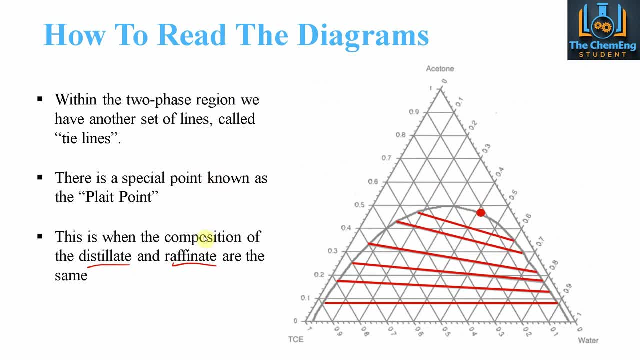 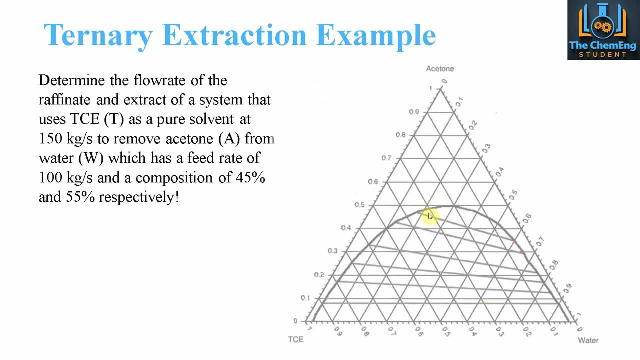 second, but essentially what we're saying is that the composition- because remember this is denotes equilibrium- that the composition between distillate and raffinate become the same. Now let's take a look at a working example here. So we want to determine the flow rate of the raffinate and the extract of a system. 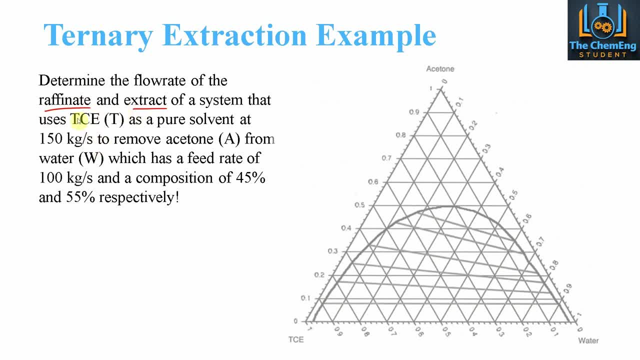 that contains trichloroethane, which we're going to denote as T, and this is pure solvent at 150 kilograms a second To remove acetone. so that's component A from water, which is component W, which is a feed rate of 100. 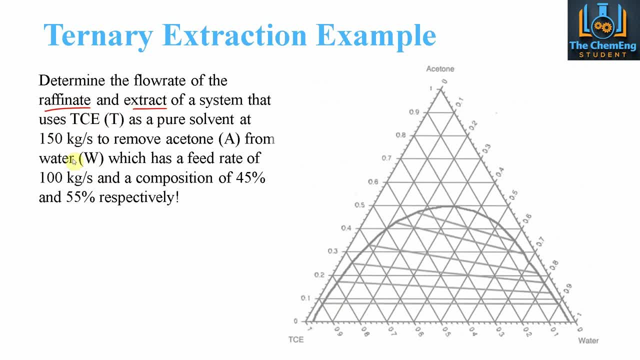 kilograms per second and a composition of 45% and 55% respectively. So, essentially, what we need to do is we need to work out the following: So if we take this as a one-stage system, so it's single-stage- we don't have multi-stage. 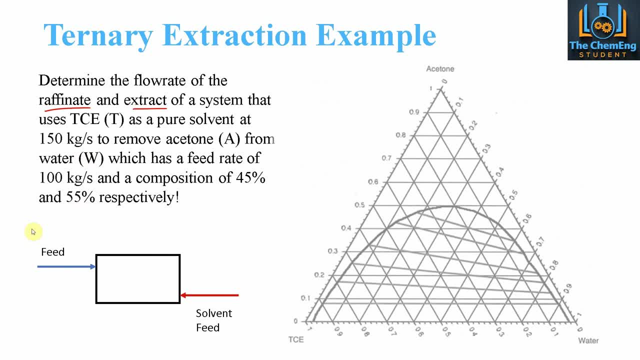 so we have the feed coming in. so that would be the one that contains the water and the acetone. and we have our solvent feed. So we have our solvent feed coming in, which is going to be our TCE. now the raffinate is: 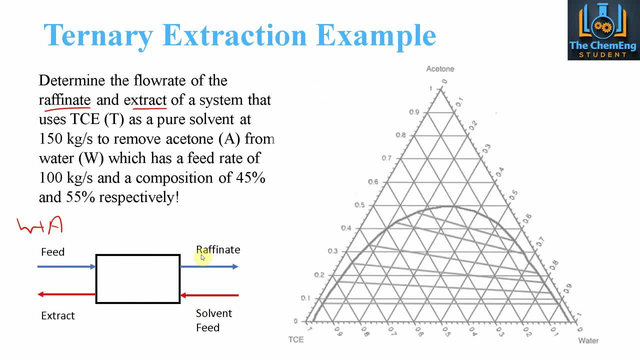 the top product. so the distillate- sorry, the extract- becomes the bottom product. Now notice that these are in counter-current flow, and that's really important so that we can improve and optimise the rate of mass transfer. It's the same principle for heat transfer. now, what's important to notice here is that 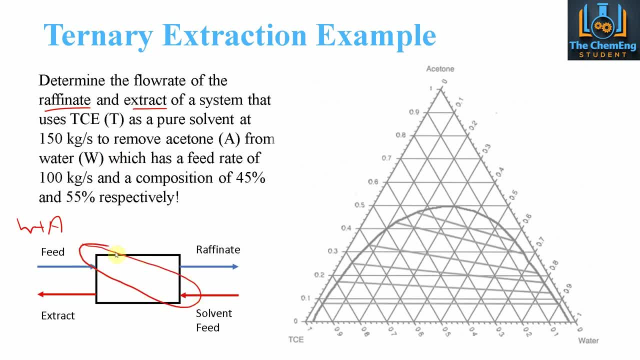 these streams are in equilibrium with each other: the feed and the solvent. Now that means that the extract and the raffinate are also in equilibrium with each other. Now, this is for single-stage. if we had multi-stage, we would just repeat the same process. 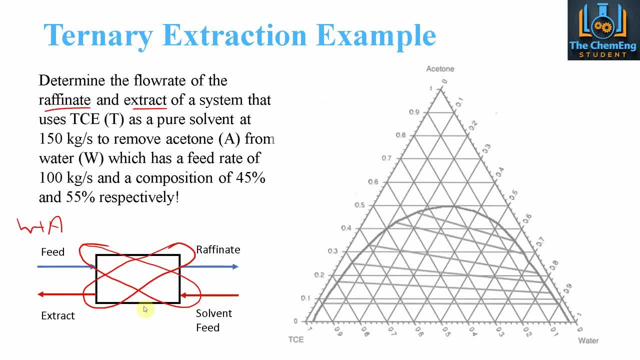 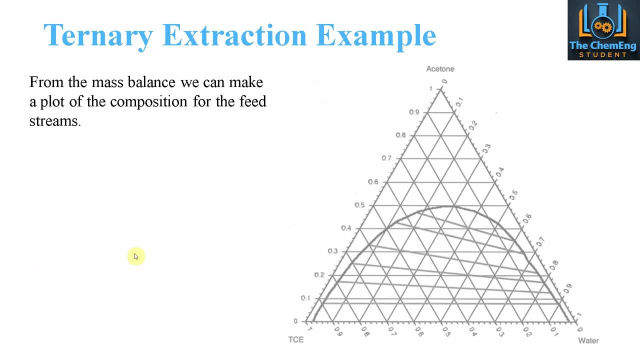 Now what we need to do here is we need to perform. so, using this as a guide, we're going to perform a mass balance on the system, and what we can do is we can make a plot of the compositions. So, to start off with, we know that the feed contains 55% water and 45% acetone, so that 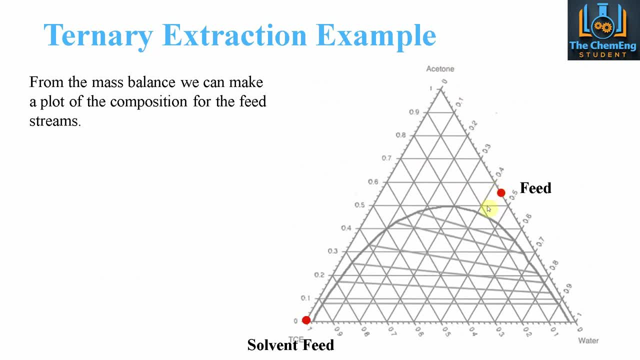 would be the feed point here. Now we know that the solvent contains pure TCE, ie we have no water and we have no acetone, so that's right down in the very bottom corner here. Now that means that we can have the feed stream plus the solvent stream is equal to this point. 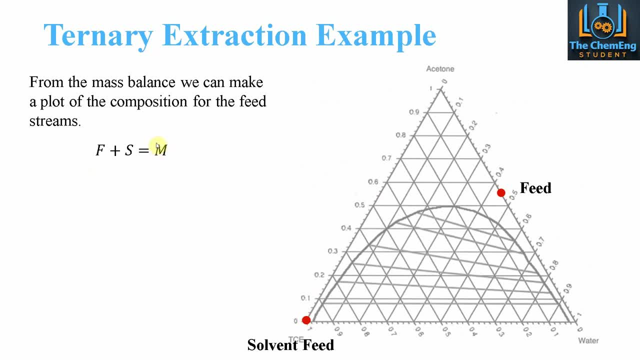 M. Now, M is the mixing point of the system and we'll come onto that in just a second. Now we can determine what M is in regards to flow rate, because that's going to be the total, so that's going to be the flow rate of the feed plus the flow rate of the solvent. 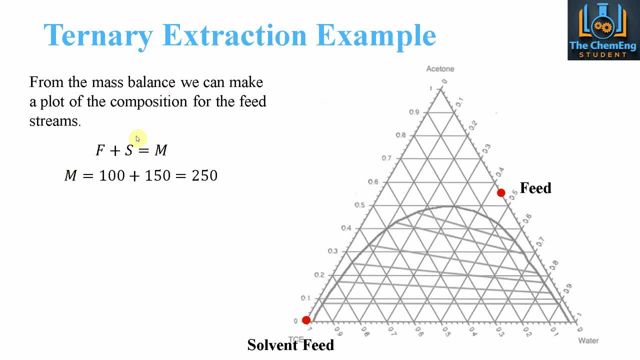 so that means that M flow rate is 250 kilograms per second. Now we can connect these points together, so this is like our operating line. Now what we need to determine is the values. Okay, so that the composition of the mixing stream so at m, and the way that we do this is we perform. 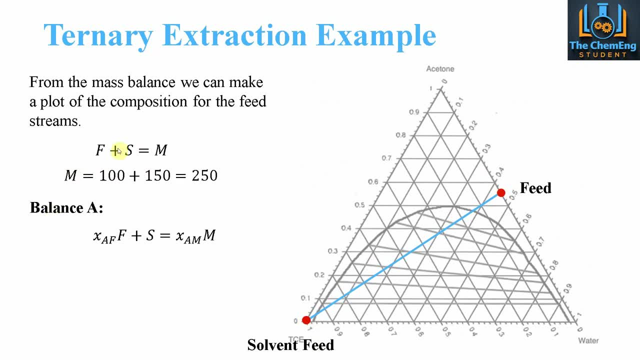 individual balances. so we'll balance the acetone first. so we'll say what is the composition of the acetone and the feet multiplied by the flow rate. now we don't have any acetone in the solvent stream, so we can just disregard that, so that will disappear. and then we have the composition of. 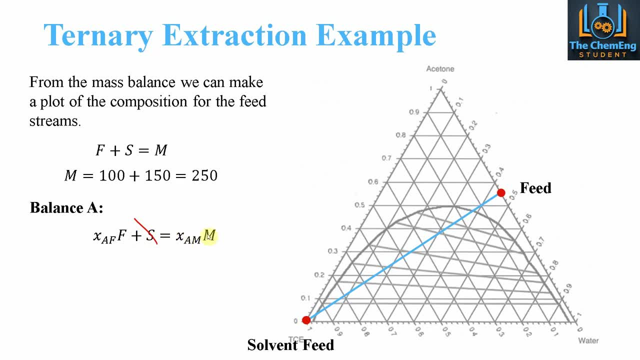 acetone and the mixing point- this is the thing that we want- and the flow rate at m, so we can pop everything in and we work out that at this mixing point and the composition of the acetone is 0.18 or 18 percent. now we just repeat the same process, but this time we'll do it on the water. 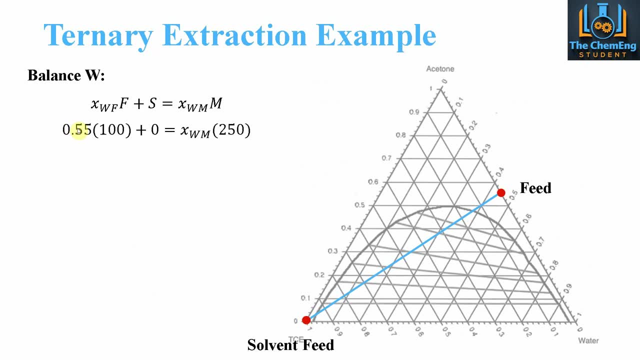 so we know that the water constitutes 55 percent. so we'll times that by 100 and then we'll divide that um 250 by that value, so that tells us that we have 20 percent water at the mixing point. then what we can say is that the remaining, so the balance for 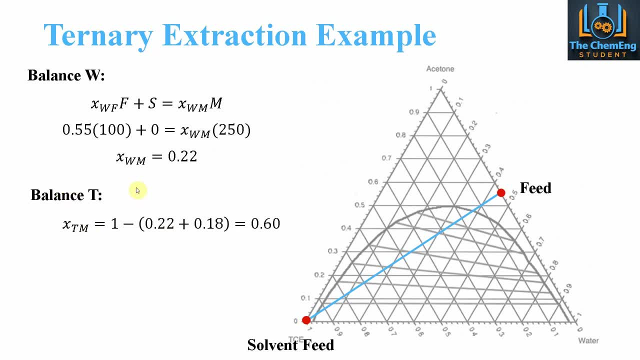 m. the trichloroethane would be one minus the summation of the, the composition of the water plus the composition of the acetone. so that tells us that we have 60 percent tce at the mixing point. now these are the coordinates for the mixing point, so all we need to do is identify. 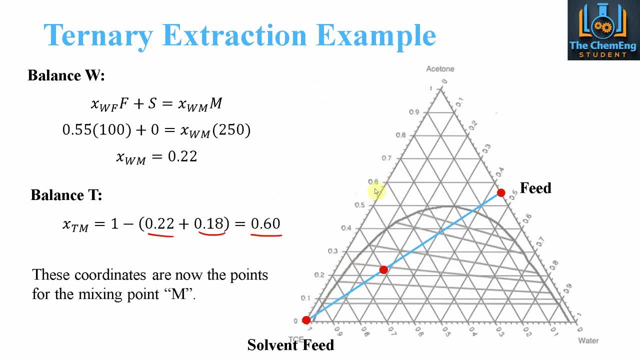 the water composition of the acetone and the flow rate at the mixing point, and then we'll specify whereabouts on the graph these lie. so we can see that our mixing point- now our mixing point- must lie on this line. so there is going to be an inherent slight error here, because we're 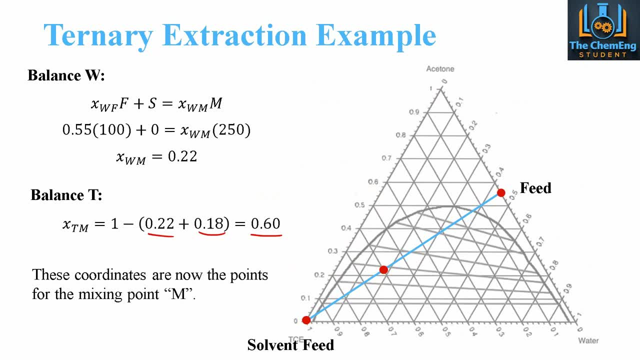 using the graphical representation. so it's open to interpretation ever so slightly, but so long as it's within a acceptable tolerance. so, for example, we know that tce is 60 percent, so we would go along. this is 90 percent, 80 percent, 70, 60, so we know that it must lie on this line. now we can clearly see that this is the point, that it's. 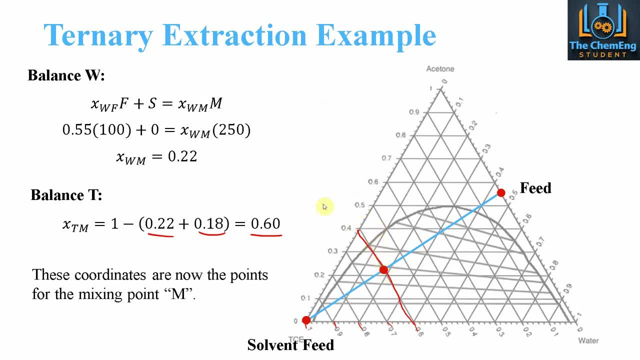 going to be, but we can get some confirmation on that because we know that, say, for example, the, the acetone or that will go for the water. the water is around 22 percent, so we go the water here. so it would be 0.9, 0.8, 0.7, 0.6 all the way up to 0.2. now we can see that it's about here. so if 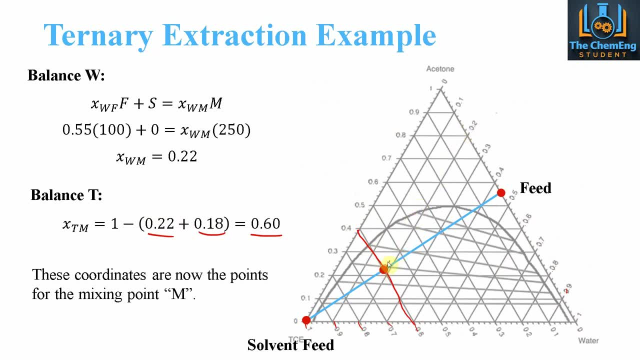 we draw a line all the way down, we can see I mean it's not going to be straight, but you get the, the general idea. we can see that will intersect there. and if we perform the same thing, you can see there is a slight tolerance of error. but we are on the operating line, which means this is our point M. so 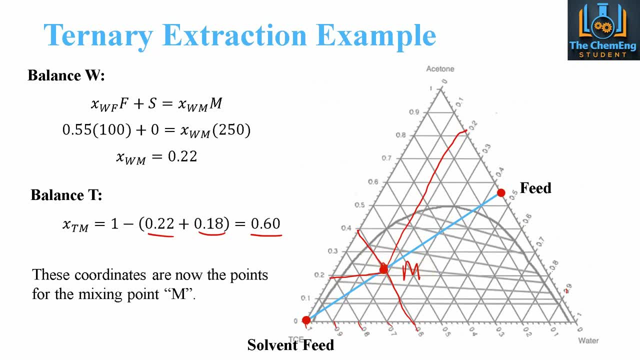 this is the mixing point, and now we know we do indeed have a two-phase system. now we need a line from point M. so remember, this is point M. now our tie lines are these lines here. so we want to be as close, we're very, very close to this line. so this is a fixed, given tiling, so we're just below. 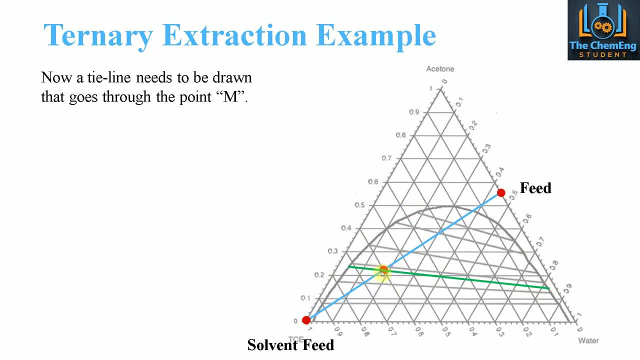 so what we'll do is we'll have, we'll match, the same gradient and we'll intersect at these points here, and these are the important points, because this is the raffinate at this point here. so to get the right, and the extract is to the left of the, the equilibrium line. now all we need to do from 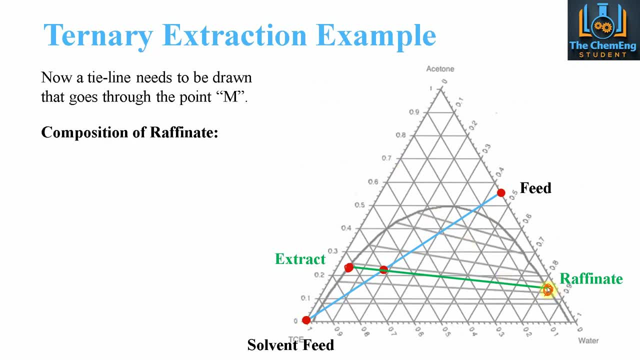 here is. we read off what the respective coordinates are for the water, the TCE and the acetone. that will give us the composition of the raffinate. so if we say that the composition of acetone and the raffinates, that's acetone and R for raffinate, is if we go all the way down here. so remember this is. 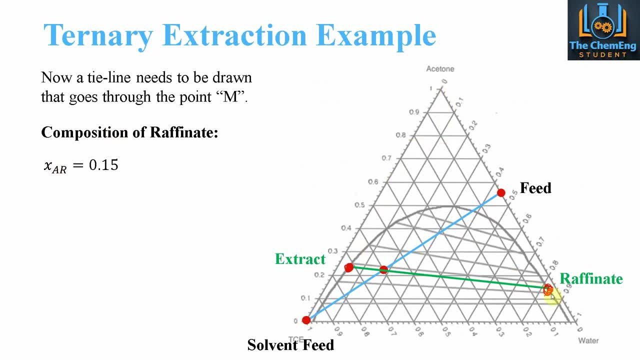 the acetone, then what we can see is that if we come down to about here, then if we go halfway and along, we can see that that's around the fifty percent mark at this point on the raffinate. so that's fifteen percent for acetone. then we could do the same, but this time for the water. so we see. 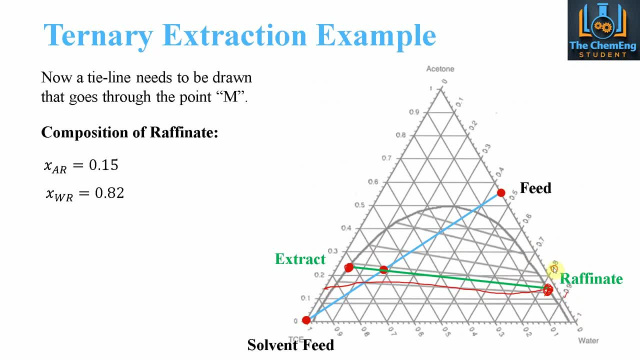 if this is pure water, then this is ninety percent water. so we're between 90 and 80 and it looks like we are just about at 82. so we say about 0.82. now the remainder is going to be these values added together and one minus that. but again, you could do the same thing here, but with the TCE, so you can. 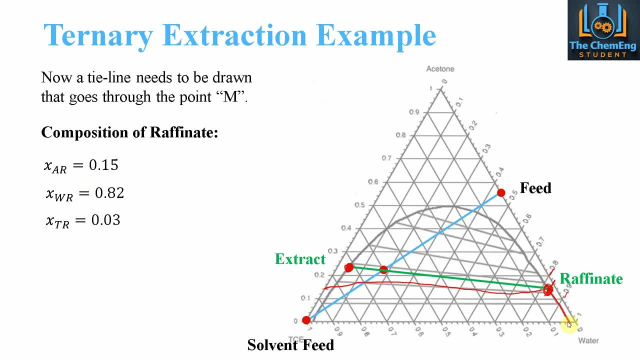 clearly see that we are on that line and we're smack bang at three, so we know that there is there is a slight error here, but we are well within the tolerance and we would do exactly the same thing. we get around 23 percent for acetone, about five percent for water and the remainder being about. 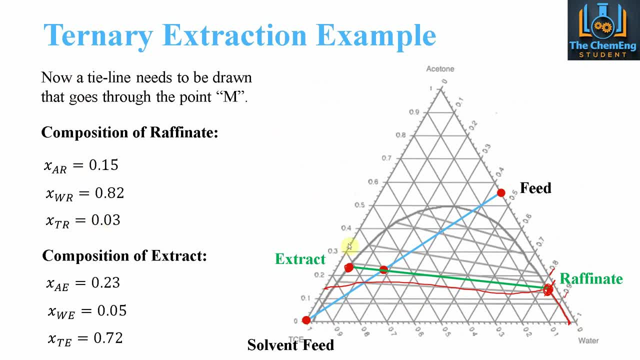 72 percent for our TCE. and again you can just double check that, because TCE here is a hundred percent and we're, we're here, so we, you know, we've got to keep the same gradient. so we're about here. so you can see that that's seventy percent, so that's 72 percent. all right, so now, from here, what? 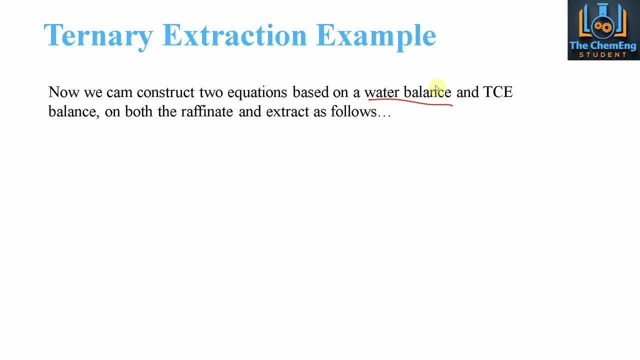 we can do is we can do this based on a water balance and we can do it on a TCE balance. so we do this so that we can determine the raffinate and the extract flow rates, because if we do a balance on the water then we know we'll have the composition, so the xwr, so that's. 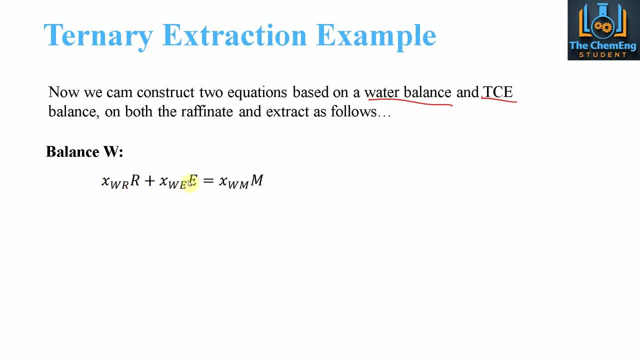 the composition of water and the raffinate plus the composition of the water and the extract must be equal to the composition of the water at the mixing point. So if we substitute in the values, then we get an equation of 0.82R plus 0.05E must equal 55.. 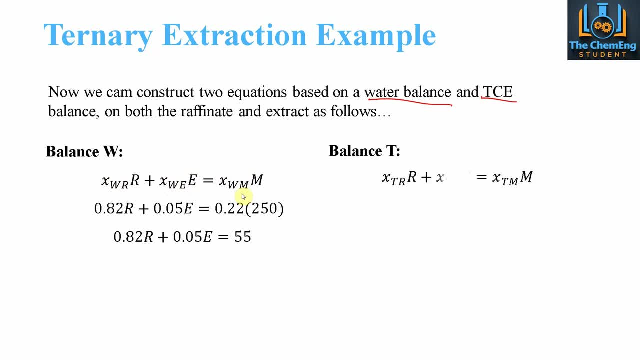 Now, if we do exactly the same thing and a balance on T, we will substitute in the respective coordinates that we achieved for TCE at both the raffinate and the extract. So we get 0.6 because we had 60% in the mixing point. 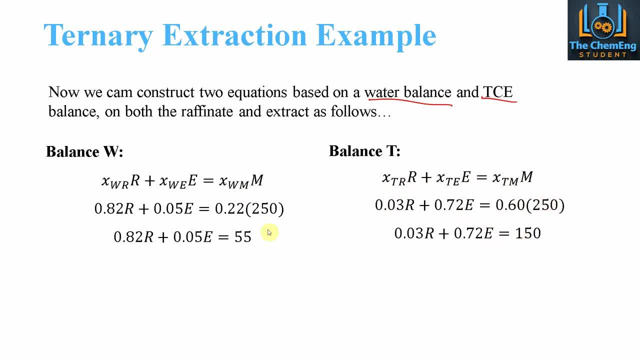 Total was 250.. So we got 150.. Now again, you could do this based on, rather than doing, M. you could say that R plus E equals F plus S, But we know that F plus S was M, So that's why we used M rather than F and S. 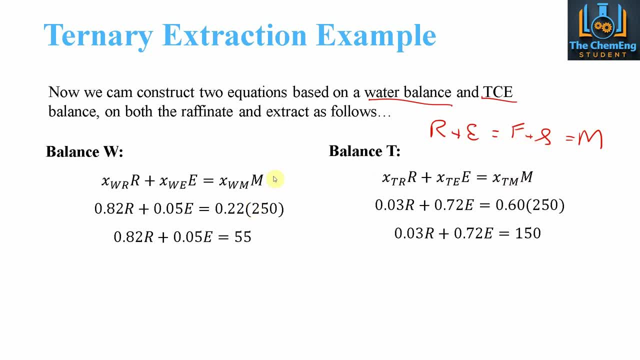 But you could do exactly the same thing and you'll get the same answer. So now, what we can do is we have a set of simultaneous equations. We have two unknowns, two equations. Now we can do this. We can do this by either elimination or substitution. 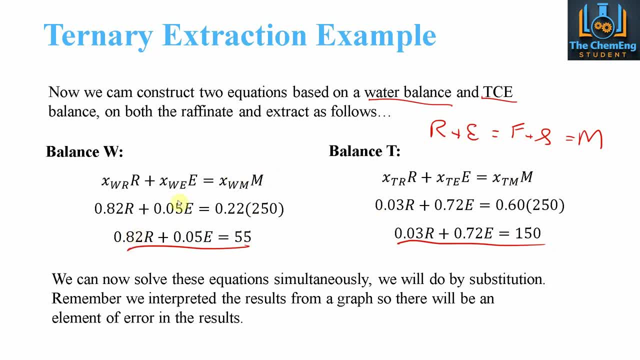 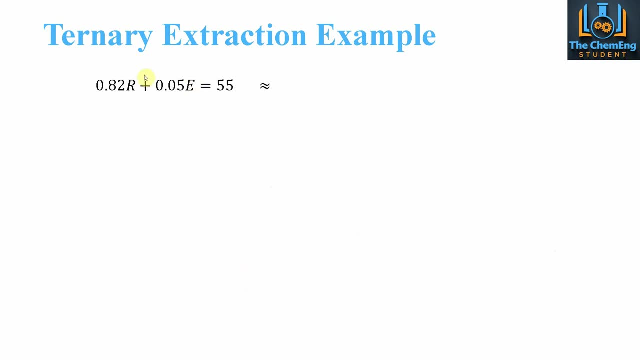 Here we'll do it by substitution, ie we will rearrange one equation and substitute it into the other. Now, just to note that we did interpret the results, so there will be an element of error within the values. So what we'll do is we'll rearrange this equation for R in terms of E. 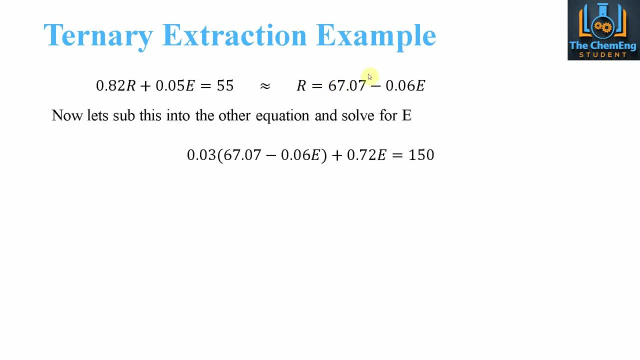 And now, what we will then do is we'll take this equation and substitute it in for R in the second equation. So therefore we've replaced R as a function of E. So then all we would do from this point is we would multiply this bracket out.